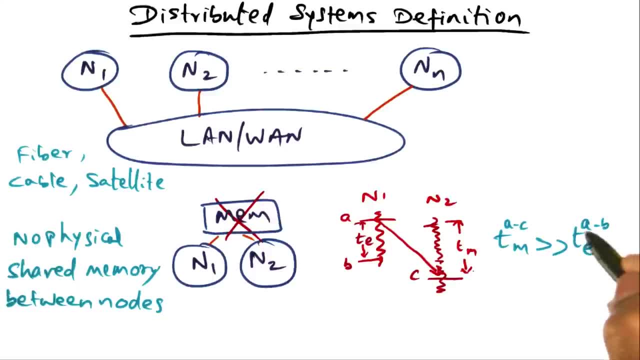 in the system, TM is much more significantly larger than the event communication time. So these are the three properties which I would like to think of to make sure that we have a shared understanding of what we mean by a distributed system, that they are connected by some sort of a local area. 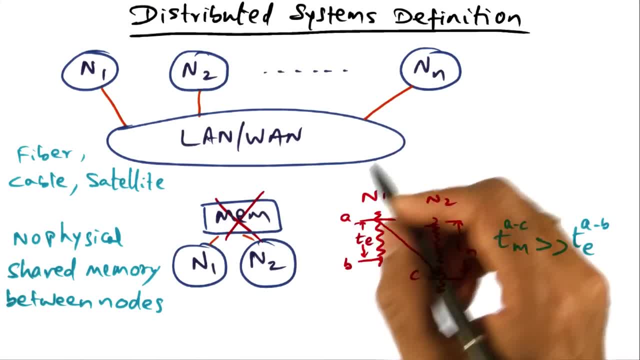 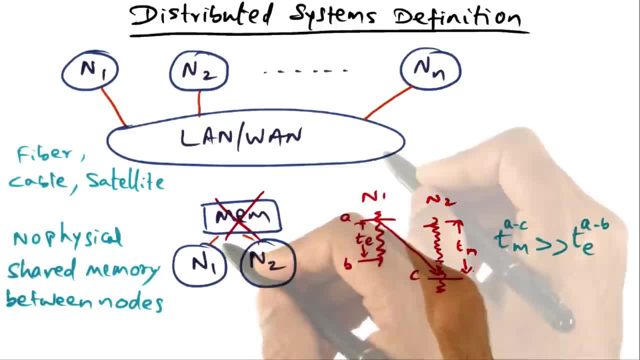 network or a wide area network, A collection of nodes, And they don't physically share memory. so the only communication, only way they can communicate with one another, is via messages that are sent between the nodes using the local area network And the third. 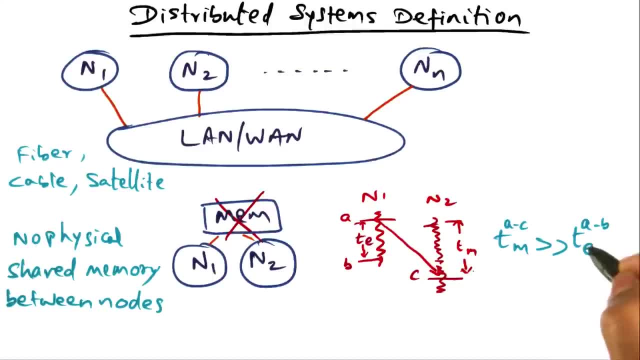 property is the fact that the message communication time is significantly larger than the event computation time that happens on a single node. You probably remember our good friend Leslie Lamport. I introduced you to him when we talked about parallel systems and I said that we will see him again In parallel systems. he's the one who gave us the 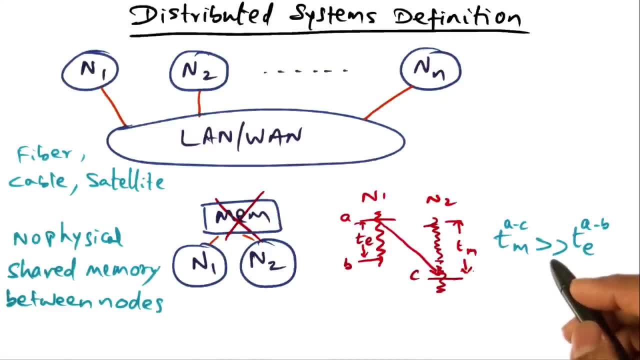 notion of sequential consistency, And he's the same person that we're going to be talking about in this lecture, Leslie Lamport, And in particular Lamport, has a definition for a distributed system, And the definition of a distributed system verbatim goes like this: A system is distributed if the message 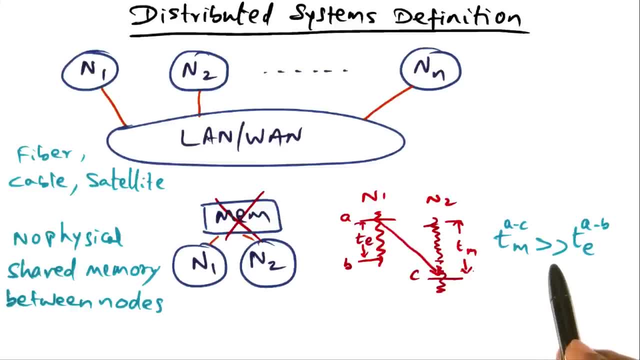 transmission time TM is not negligible to the time between events in a single process, So there's a time between events in a single process. there's a message transmission time, And so the definition that Leslie Lamport gives is that a system is distributed if the 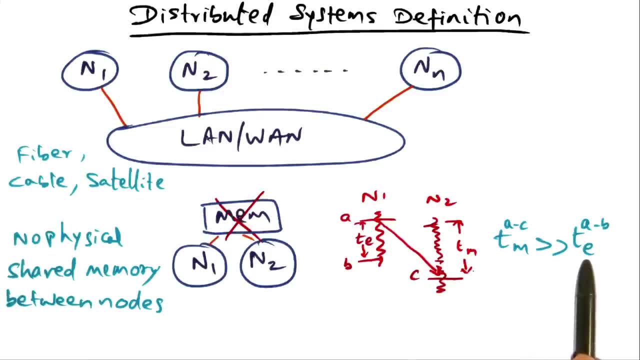 message transmission time TM is not negligible compared to the time between events in a single process. What is the implication of this definition? Interestingly, even a cluster is a distributed system by this definition. We've been talking about clusters a lot when we discuss parallel systems and I told 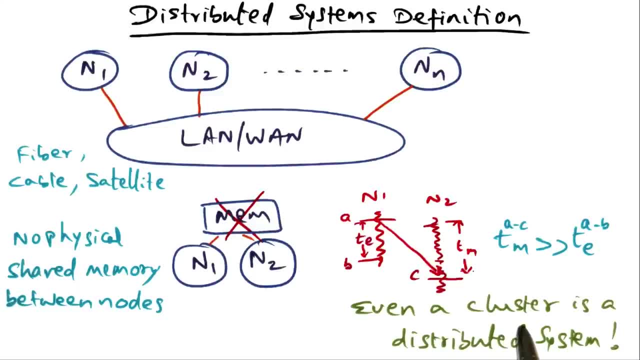 you that clusters are the workhorses of data centers. today, Even a cluster is a distributed system by this definition, because processors have become blazingly fast, and so the event computation time has shrunk quite a bit. On the other hand, the message communication time is also becoming better, but not as fast as the 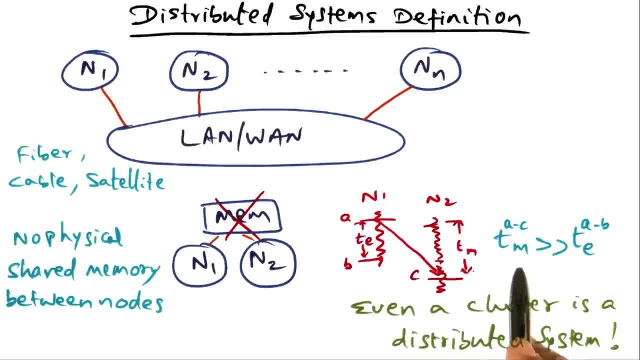 computation time. that happens on a single processor And therefore even in a cluster, which is all contained in a single rack in a data center. the message transmission time is significantly more than The event time, And so even a cluster is a distributed system by this definition. The importance of this inequality is in: